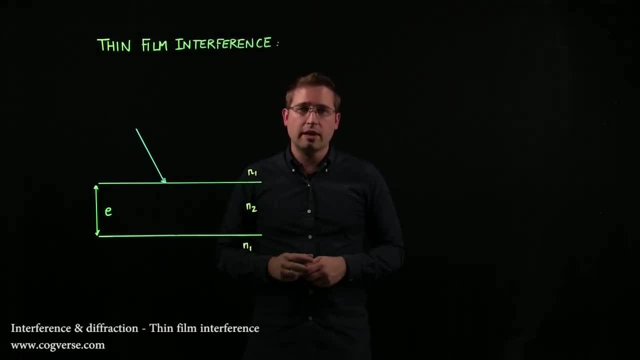 Thin film. interference occurs when light is shined on a very thin film of soap, for example, and the reflected light from the different surfaces of the film interferes constructively or destructively. It's a very classic problem, but it's a bit hard to set up, so we're going. 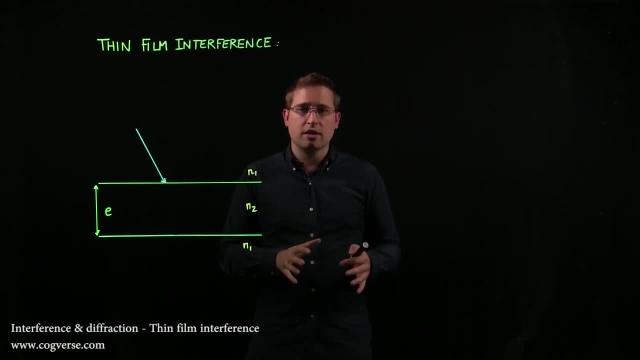 to spend some time on the drawing and on deriving the equations that give you constructive or destructive interference. Let's consider this film here. Let's say it's a film of soap, just to get a visual fix on it. and this film has a thickness E that is very, very. 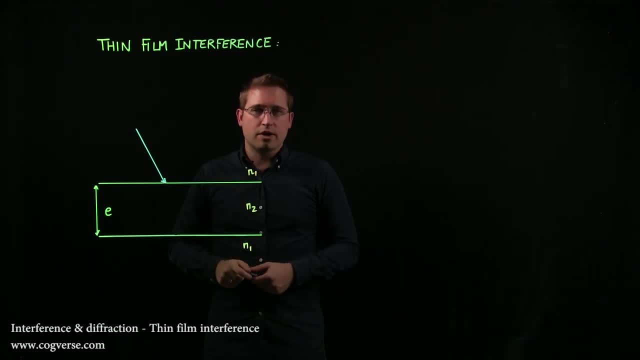 small, of course, and we are going to shine some light onto this film. Now. we know that if light hits this surface, it's going to be reflected and probably going to be refracted as well, and it's going to enter the film. Now, probably, these rays are close to vertical. 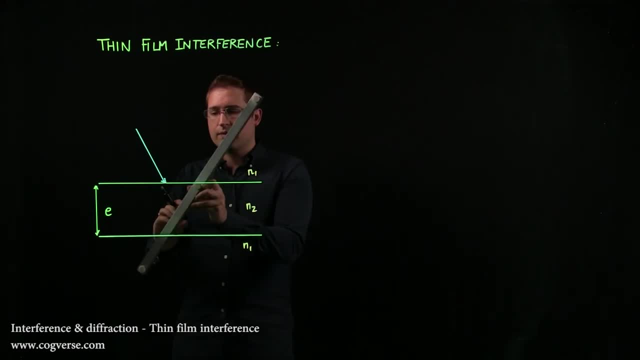 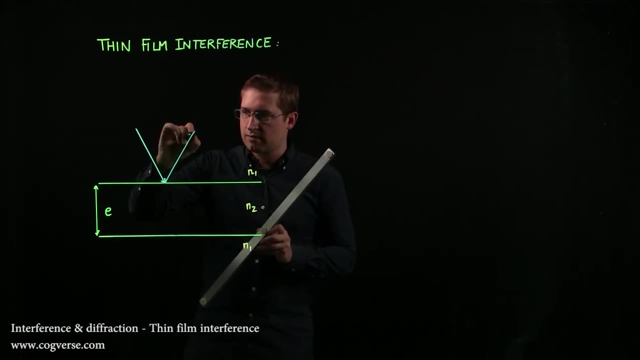 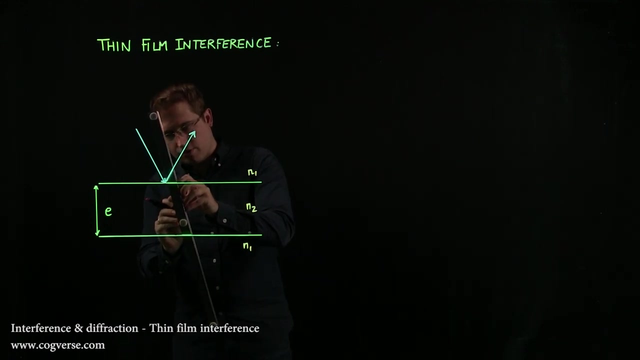 but I'm going to exaggerate them so that we see what's going on. I'm going to draw the reflected ray off the film like this, and the refracted ray is going to enter the film, and I'm going to exaggerate things, but let's just draw it like this, just. 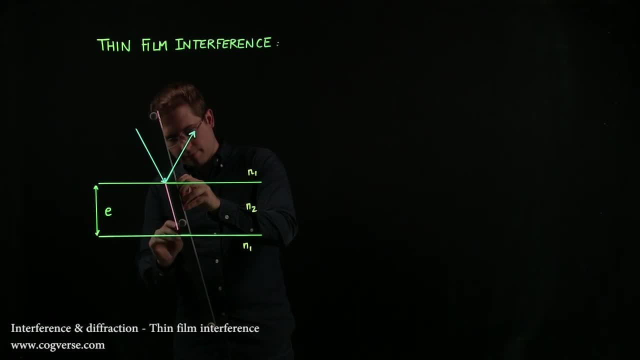 to again understand what's going on. Here's the refracted ray, and now that it hits this interface it's probably going to be reflected off of it and then it comes back up. It hits this interface and then it refracts out and it comes out pretty much parallel to this. 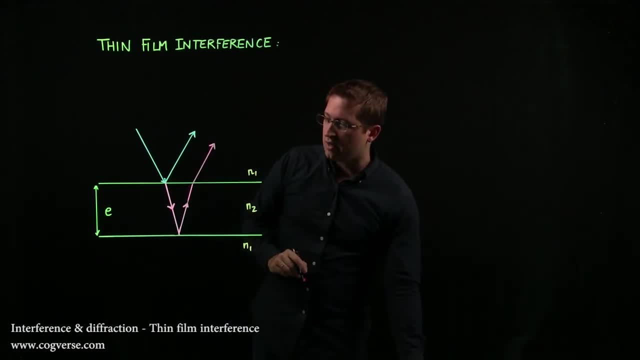 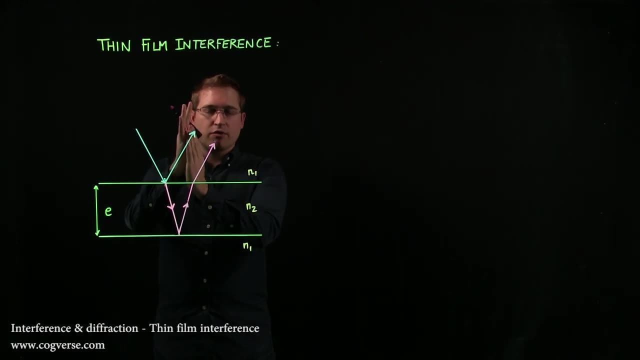 guy here. Now I've exaggerated everything, all the angles, but think of these rays as being pretty much collapsed into one. So I'm going to draw a very small, big vertical pile of rays. In other words, this distance is very, very, very small. but if I make it very, very small, then we can't see what's. 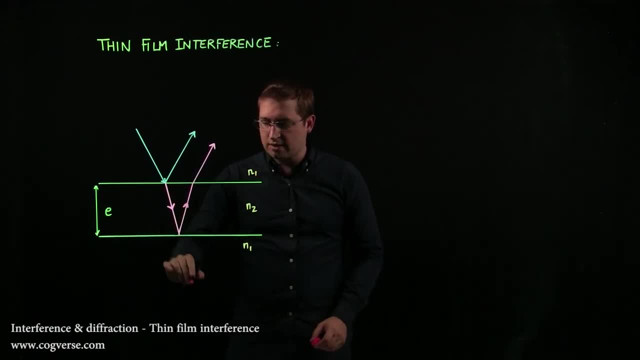 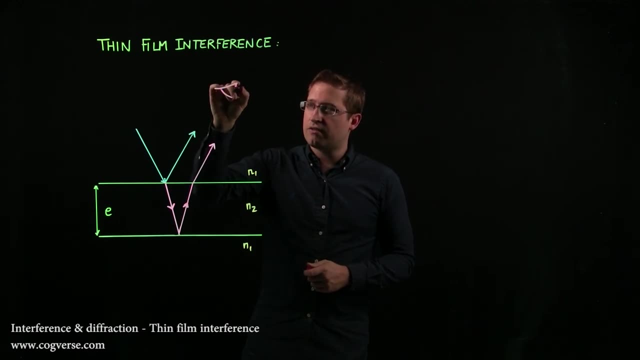 going on. Now you might say: well, wait a minute. Why didn't you draw the ray that exits the film? I could have- and there probably is one. I'm not going to draw it because I don't care. I'm going to assume that I'm looking at the film from here and what I'm going. 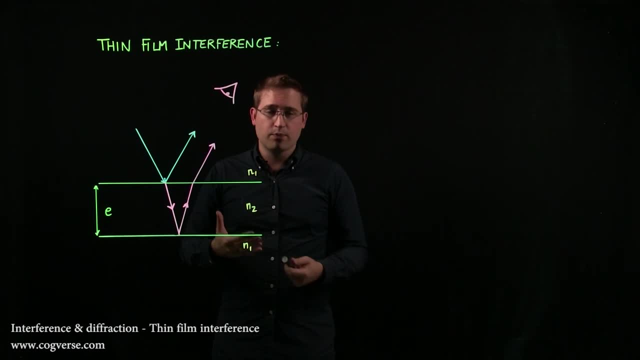 to be interested in is whether these two rays interfere constructively. Now, clearly, these two rays- the blue one here and then the red one- do not travel the same distance and therefore, when this one exits the film, it's going to be shifted by. 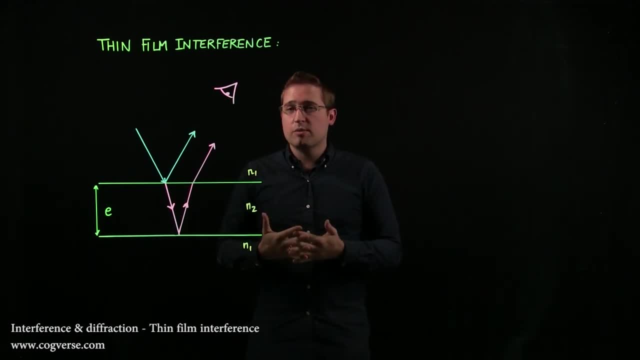 a certain amount with respect to this one. We need to be able to quantify delta X, the path length difference. We also need to take into account what goes on at each interface, because remember that we said that when wave reflects off an interface, it might undergo a phase shift. So we're going to 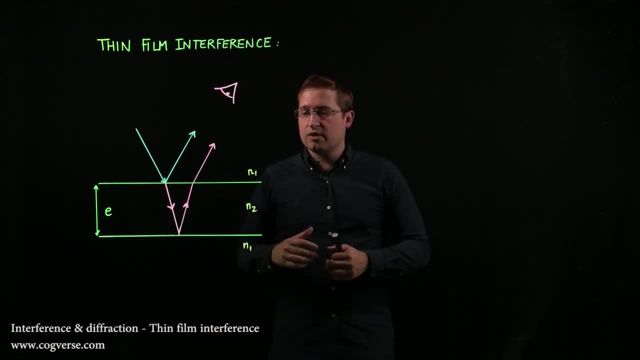 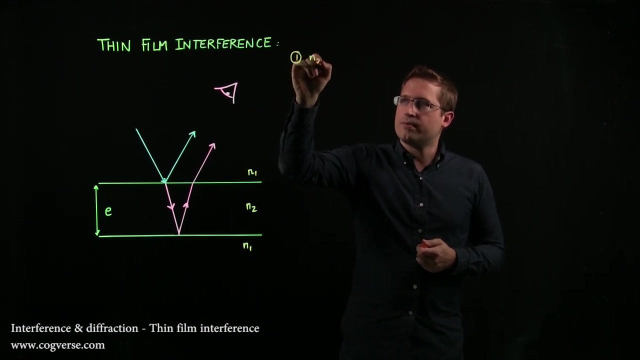 have to be very careful in doing this, and we're going to have to distinguish two cases. Either N2 is going to be greater than N1, or N2 is going to be less than N1.. So let's get started. The first case is going to be: N2 is greater. 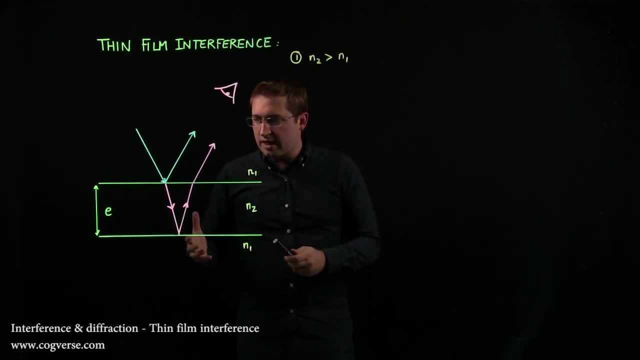 than N1.. Now, if I want to write delta x for this problem, I want to figure out what is the extra distance that this red ray traveled compared to this blue one. Well, in fact, if you look at it, the extra distance is just the back and forth. 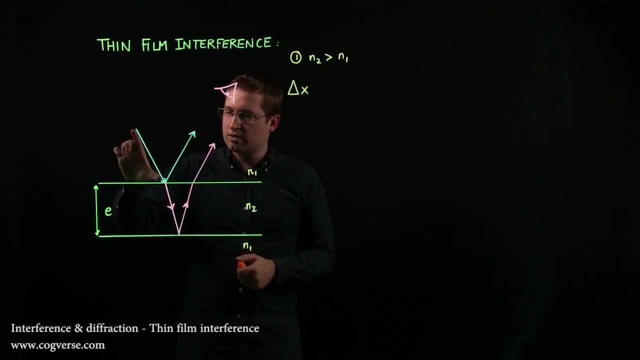 travel within the film, Because this is common to both rays, and once it exits, who cares? I want to know if they interfere, but the difference in traveling is greater than N1. So I want to figure out what is the extra distance. 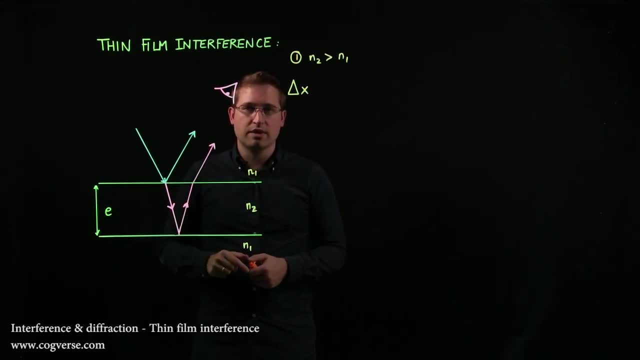 travel. is this E and E once again? Now you're going to say: well, it's not quite E because it's at an angle. That's true. Remember that I exaggerated the angles, So we can assume that this is pretty much all vertical and therefore the distance from here to here is. 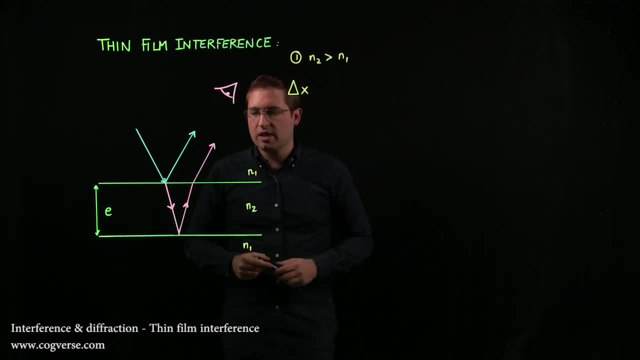 pretty much E From here to here again is E, So the difference is going to be an extra distance of two E traveled by ray. call it number two. Start labeling rays. to make things simpler, However, the blue ray here hits a surface with a greater index of refraction. 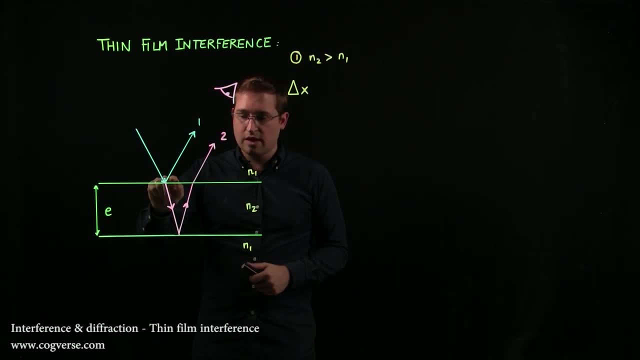 Therefore, right here I have a phase shift. I don't have one here, because N2 is greater than N1 and therefore the red ray does not get shifted when it reflects off this surface. But off this surface the blue ray does undergo a phase shift. Therefore, it is as if the 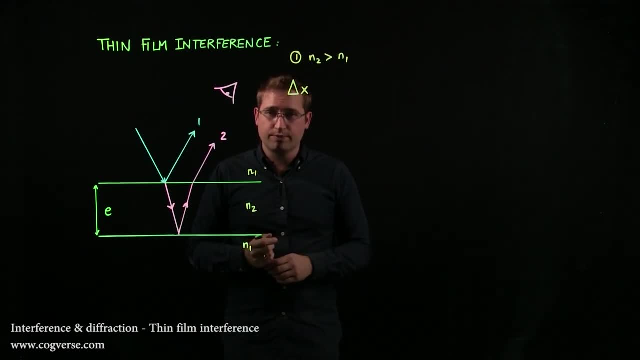 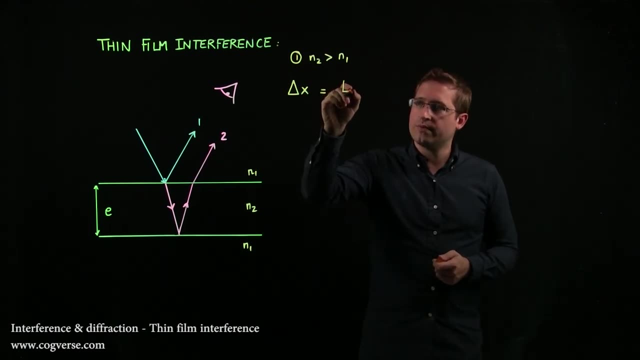 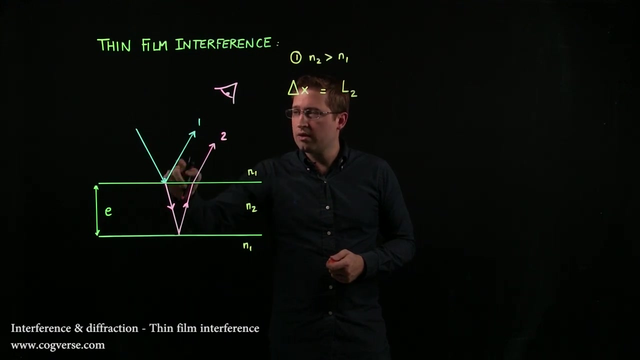 blue ray traveled an extra distance lambda over two. All right, Let's get this all into an equation. Delta X is going to be L2, the length of the path followed by the red ray, minus L1, the length of the path followed by the blue ray. 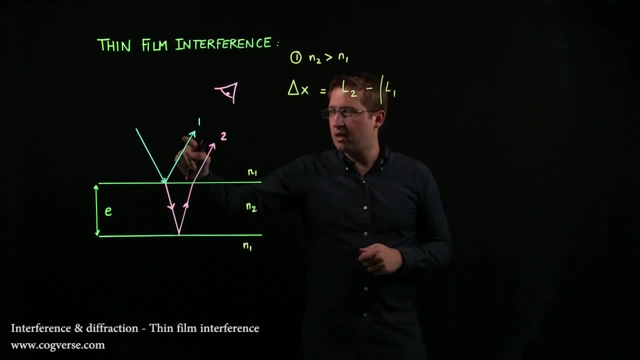 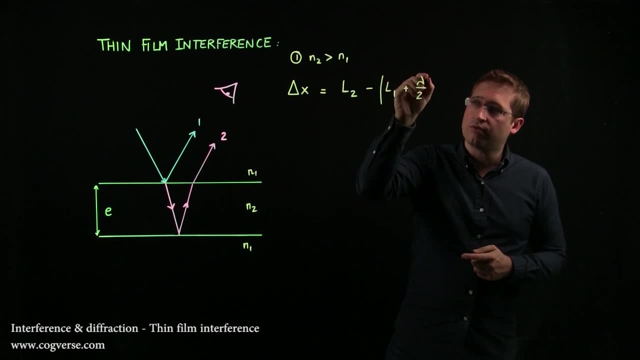 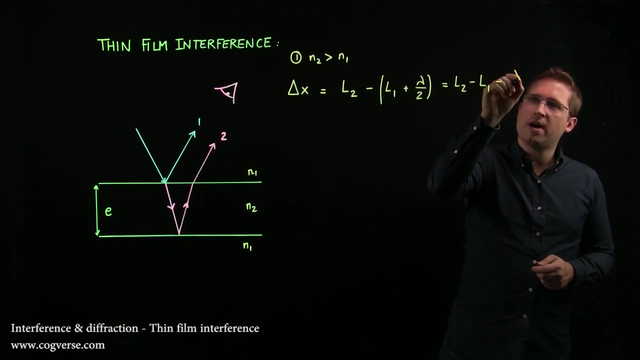 but remember that we said that because the blue ray undergoes a phase shift, here it is as if it traveled an extra lambda over two that I'm going to account for here. Therefore, I get L2 minus L1, minus lambda over two. This is usually what is forgotten, so be very careful. 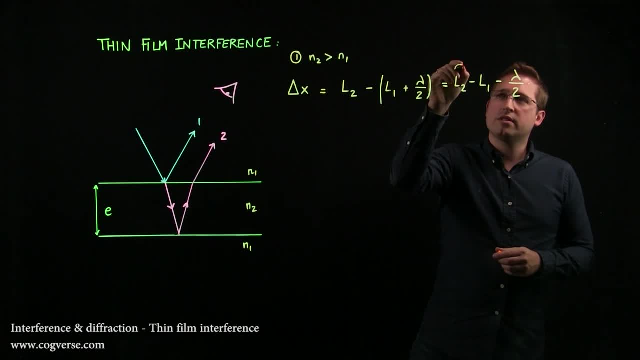 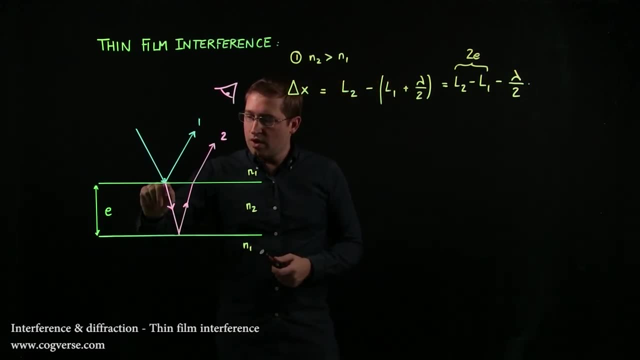 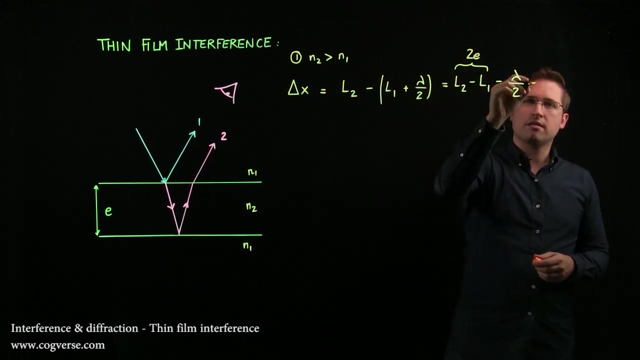 with this. This quantity here- L2 minus L1,, as we argued previously- is simply two E, because the difference in path length is one E this way, one E that way, so it's two E. In other words, my delta X is equal to two E minus lambda over two. 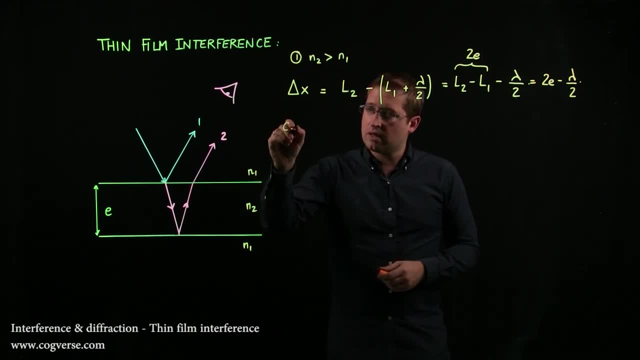 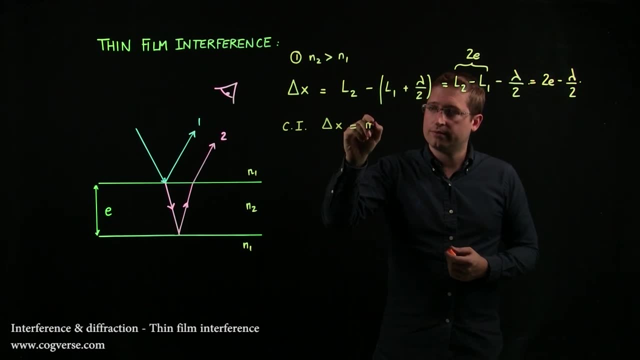 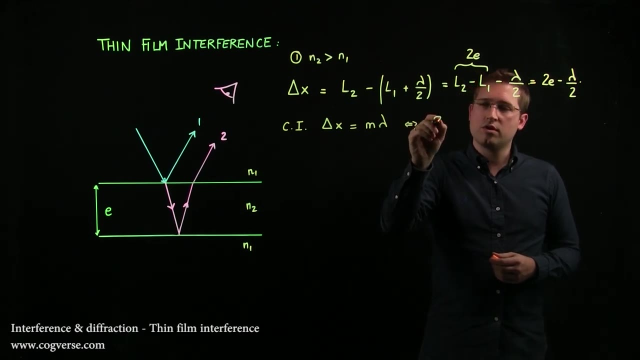 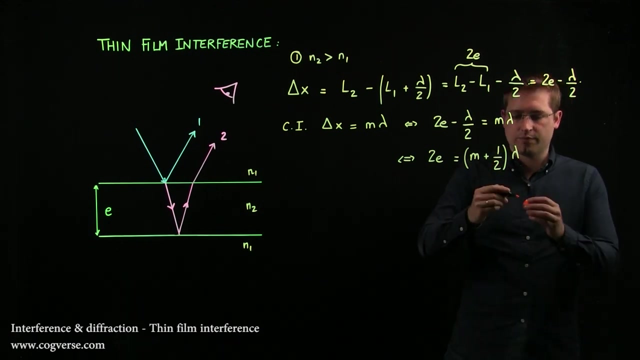 I will get constructive interference here. if delta X is equal to some integer multiple of lambda, I know that That is the same as saying that two E minus lambda over two is equal to M lambda, which is the same as saying that two E must be equal to M plus one half lambda At this point. you might wonder and say: hold on, Constructive interference is equal to two E minus lambda over two. That is the same as saying that two E must be equal to M plus one half lambda. At this point you might wonder and say: hold on, Constructive interference is equal to. two E minus lambda over two. That is the same as saying that two E must be equal to M plus one half lambda. At this point you might wonder and say: hold on. Constructive interference is equal to delta, X is equal to two E. See instead of constructive interference. 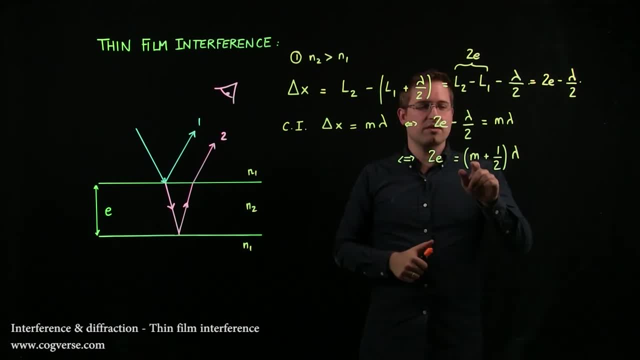 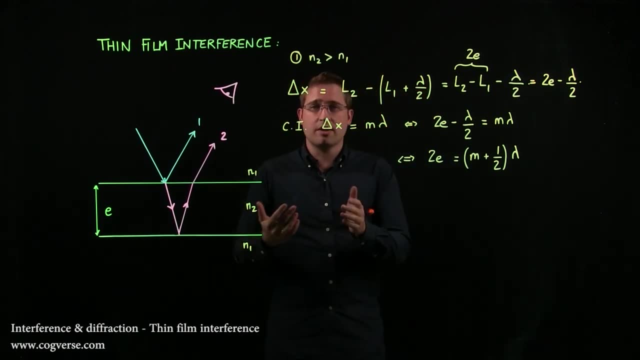 I get M plus one half really, Because this's 1.5 wavelengths or 2.5, or 3.5.. I thought that when delta X was equal to that, waves were shifted by 1.5,, 1.5, 2.5. 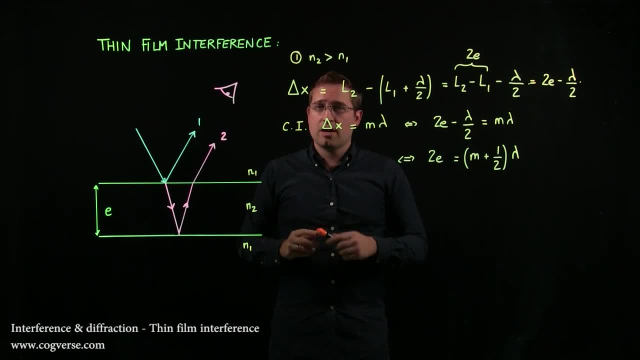 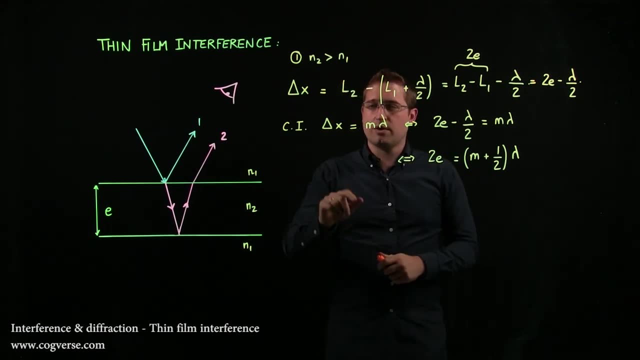 3.5 and were exactly out of phase. That's true, but careful, This is not delta X, this is two E. See, we said what we had to say for constructive interference here. We said: delta X equals M lambda. 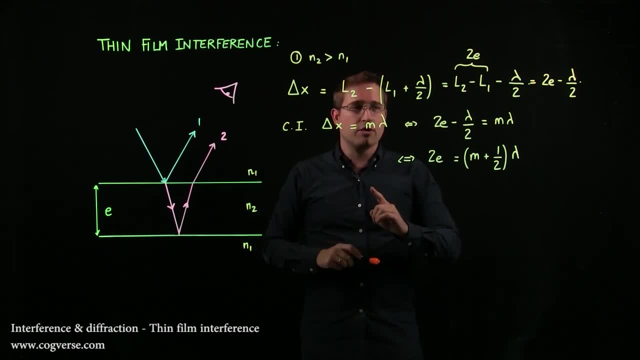 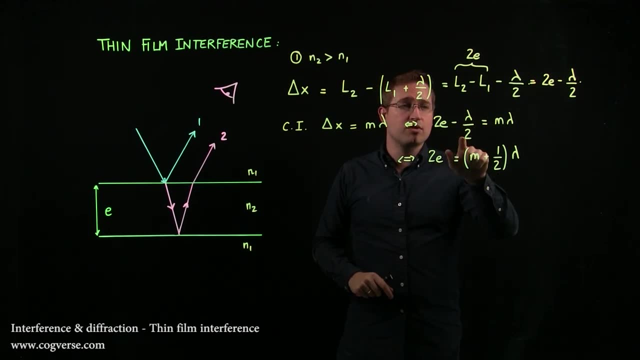 unequivocally- is constructive interference. However, because of this lambda over 2 that came from the phase shift on this surface I have 2e minus lambda over 2 equals m lambda, which in the end gives me this: In other words, for a given thickness of a film, there is a given lambda. 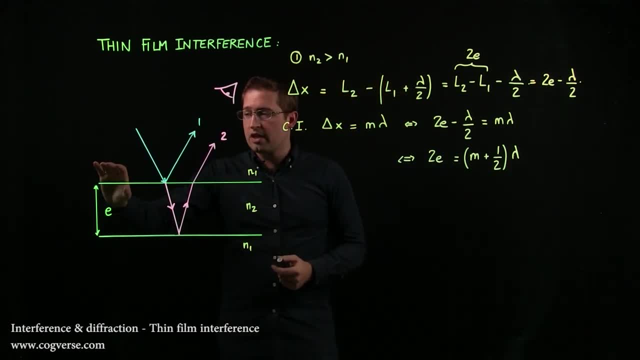 and that means that I will see different colors if the film thickness changes, and that's what happens in bubbles, for example. In a bubble, the film is heavier at the bottom because the fluid goes down to the bottom. therefore it's thicker, and you don't see the same colors on top than at the bottom. 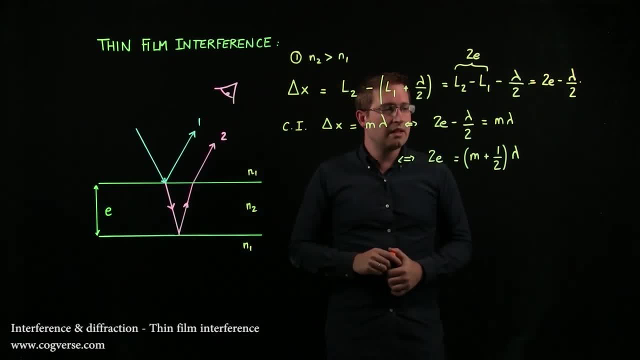 That's because the film thickness changes. So, that being said, the condition for constructive interference is delta x equals m lambda, and that yields 2e equals m plus 1 half lambda. Don't let the fact that it looks like destructive interference throw you off. 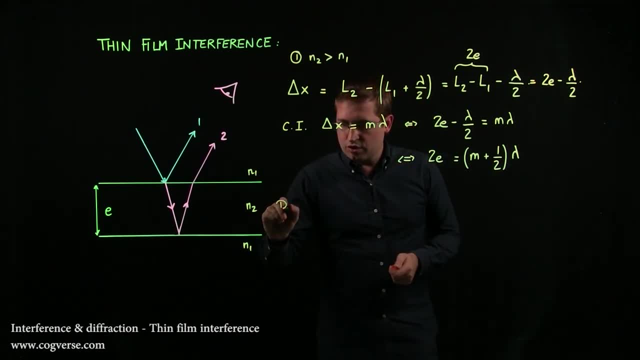 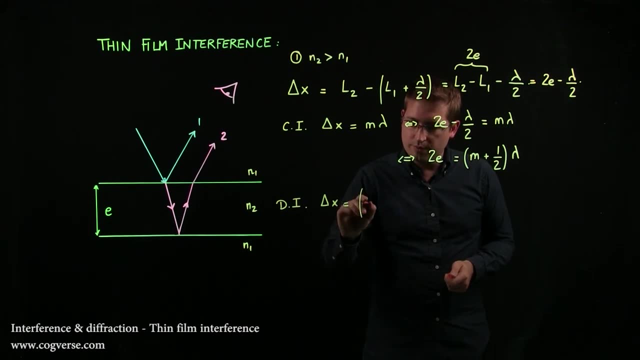 That comes from the phase shift. Of course we should do destructive interference as well. and that is: delta x is equal to m plus 1 half lambda. right, So it looks like it, but this is the actual condition. This was constructive, this is destructive. 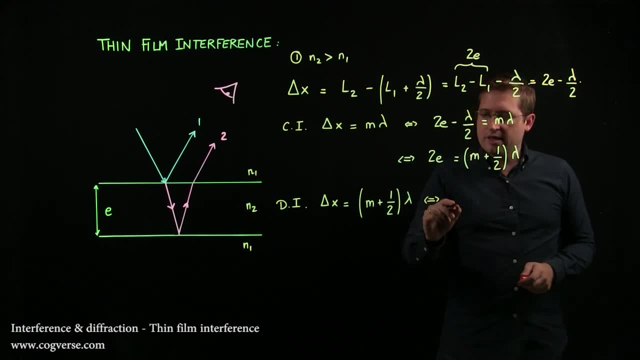 And now if I write this, then it's the same as writing: minus lambda over 2 is equal to m plus 1 half of lambda, which is the same as saying 2e is equal to m plus 1 lambda, because lambda over 2 plus lambda over 2 gives me 1.. 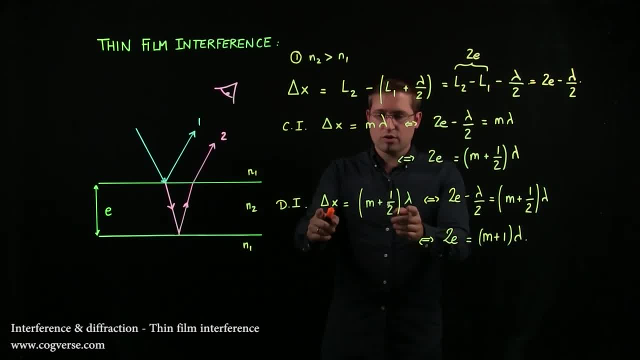 And again, this looks like constructive interference, but it's not. It's destructive. because of this, It's simply the phase shift that we have. We have to look at this interface that makes the result look different. So what's important is that you understand how we got to this. 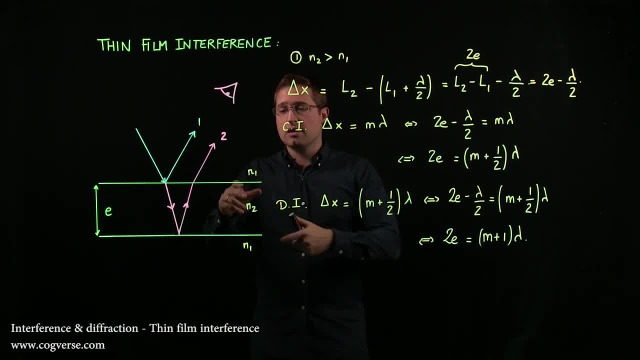 I don't even really care if you memorize this- You probably shouldn't because you might not be in the case n2 greater than n1, but I care that you understand that the condition for constructive interference is delta x equals m- lambda. The condition for destructive interference is delta x equals m plus 1 half of lambda. 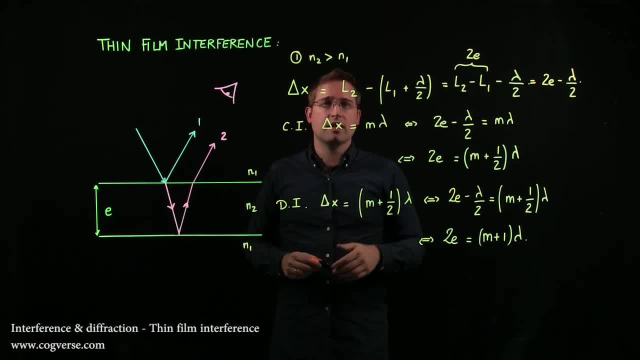 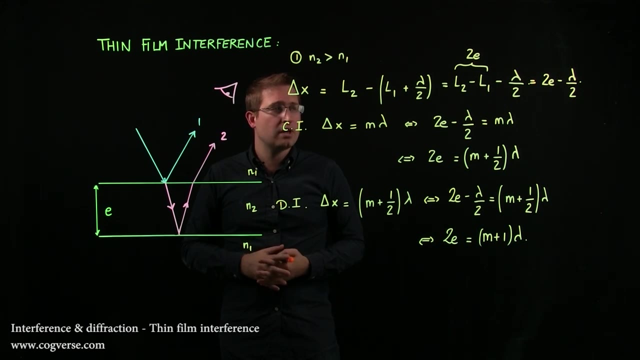 and then you just have to find delta x, And here delta x is the difference in path length, which is physically 2e. But you have to account for the fact that here at this interface, it is as if the blue ray had traveled an extra lambda over 2.. 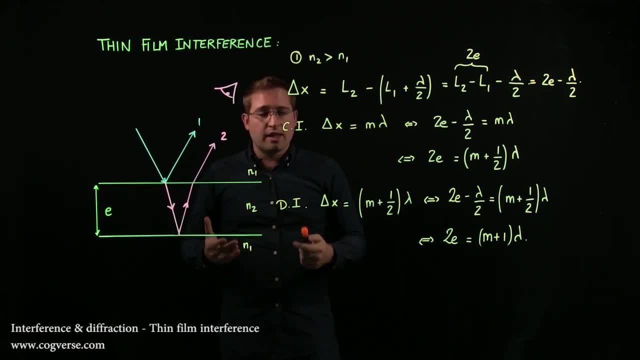 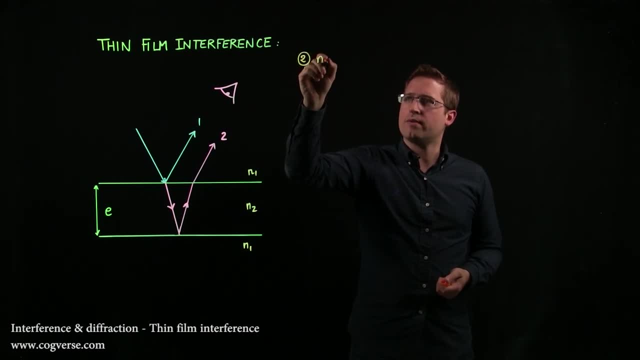 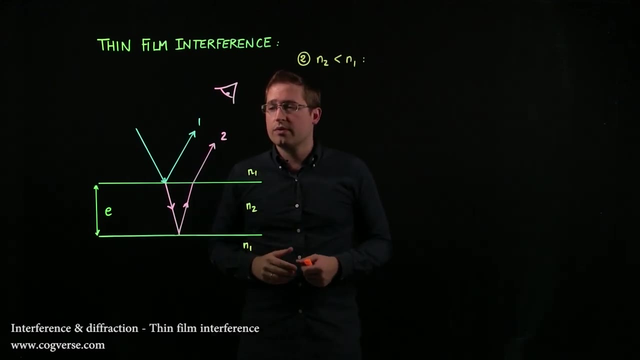 So this is for n2 greater than n1.. Let's do n2 smaller than n1. Now, if n2 is smaller than n1, what changes? What changes is that? now the blue ray reflects off a surface with a lower index of refraction. 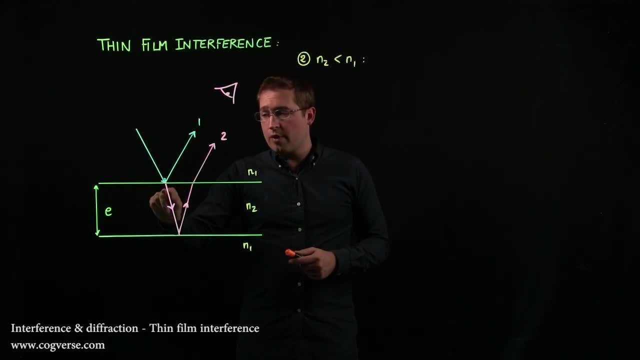 and therefore does not undergo a phase shift. However, the red ray undergoes a phase shift here, because n1 is now greater than n2.. So there still is a phase shift, but it's a different ray that undergoes that phase shift. 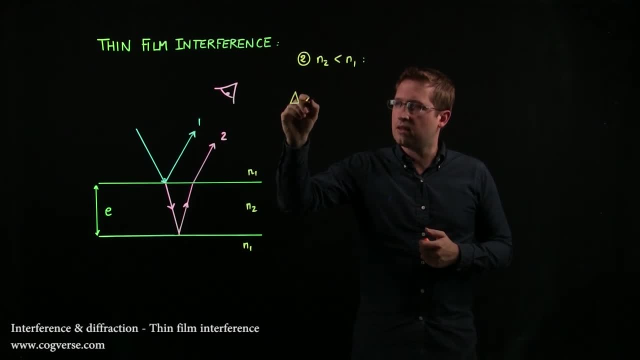 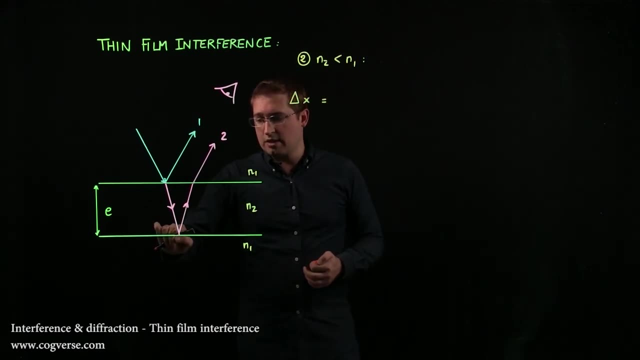 So let's find delta x. Delta x is equal to l2 minus l1, basically, However, I have to account for the fact that there is now a phase shift here and that it is as if the second ray had traveled an extra distance, lambda over 2.. 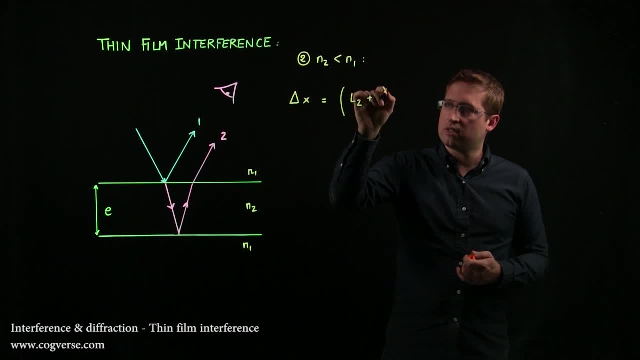 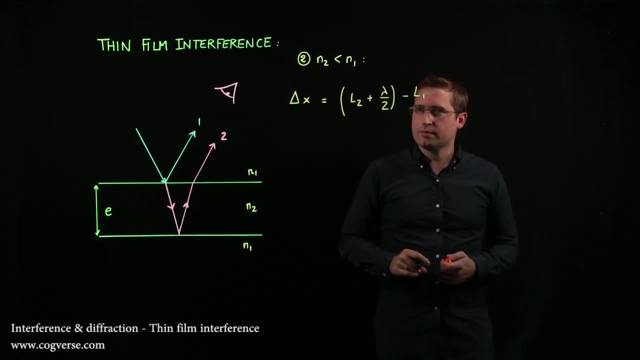 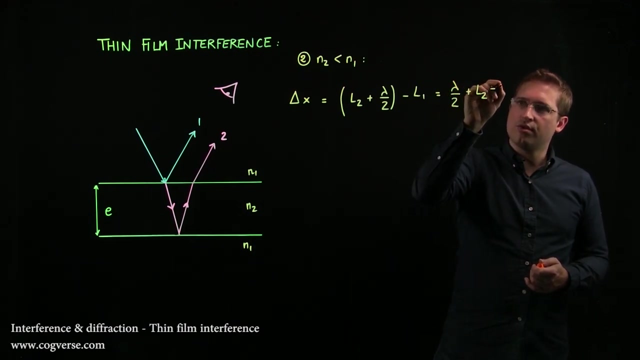 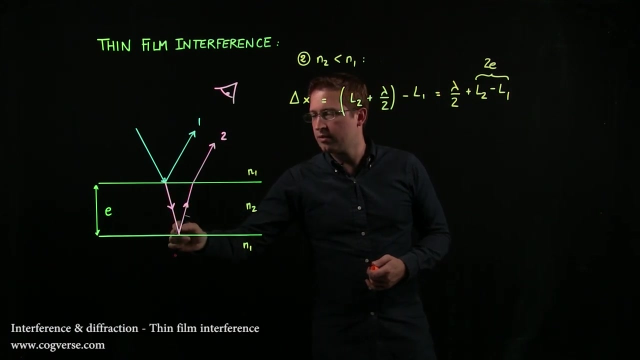 Therefore I write l2 plus an extra distance, lambda over 2, minus l1. And that is lambda over 2, plus l2, minus l1. And physically speaking this again is 2e, 1e this way, 1e this way. 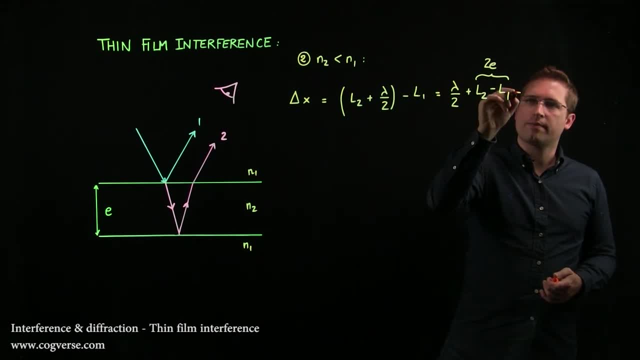 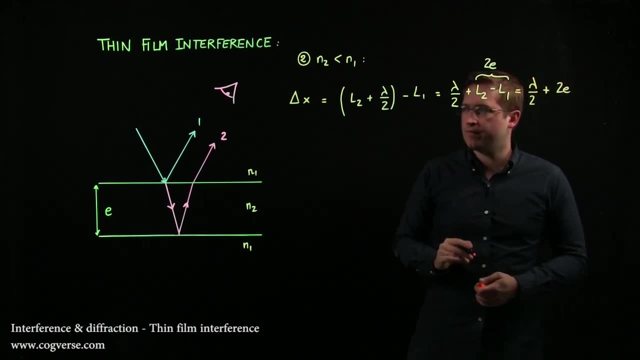 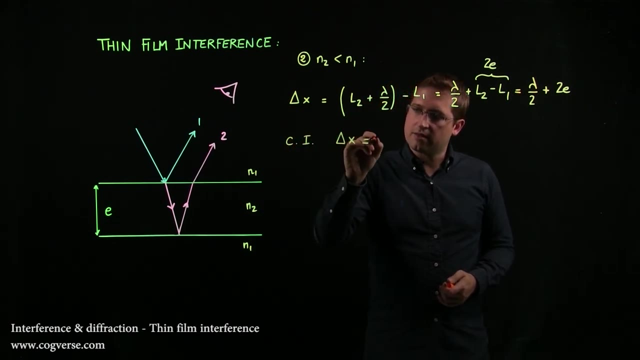 That is really the physical path length difference And therefore I get lambda over 2 plus 2e. Now if I want constructive interference, I write that delta x must equal m lambda, because then the waves are shifted by an integer multiple of wavelengths. 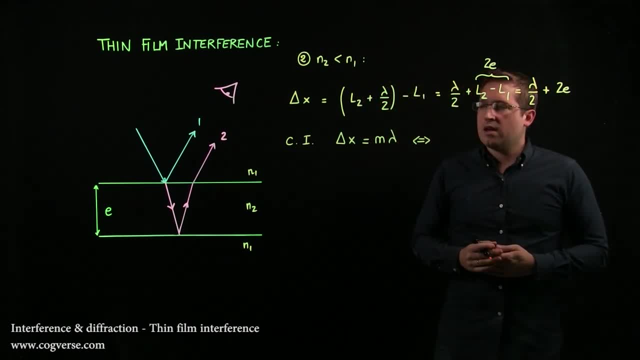 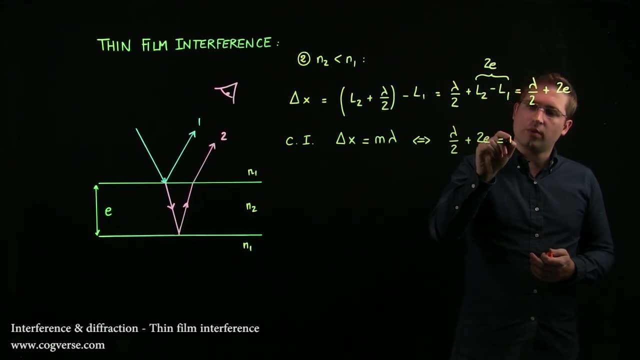 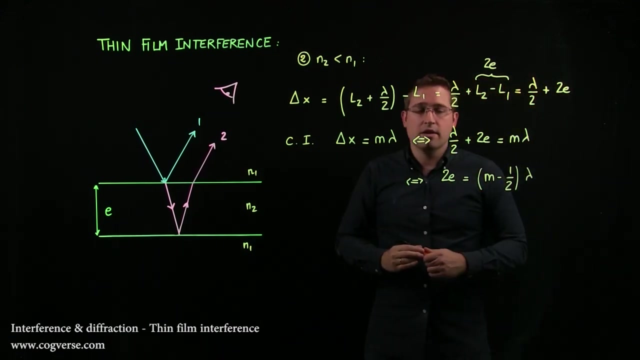 and I get constructive interference. That is the same as writing: lambda over 2 plus 2e is equal to m lambda, which is the same as saying 2e is equal to m minus 1 half of lambda. Once again, this looks like a destructive interference condition. All right, 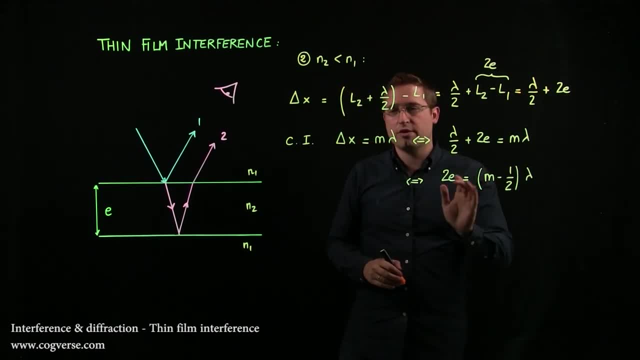 But it isn't. It is the result of having said I want constructive and having a phase shift at this point here that we accounted for, which is lambda over 2.. So this gives us constructive interference and any wavelength that satisfies this equation. 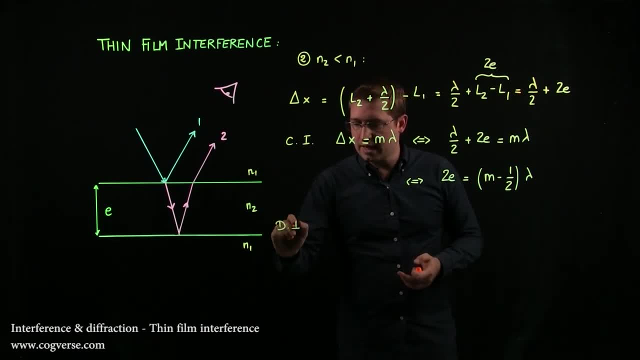 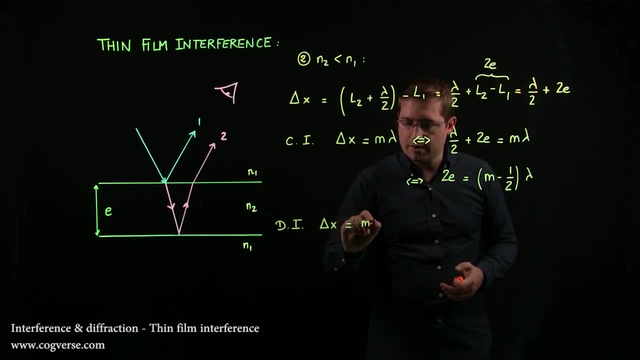 will interfere constructively. To get destructive interference, I write that the condition is to have delta x equal to m plus 1 half of lambda, which, by the way, is the same as 2m plus 1 times lambda over 2.. 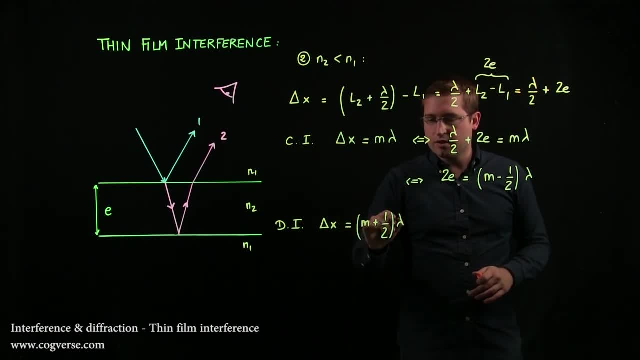 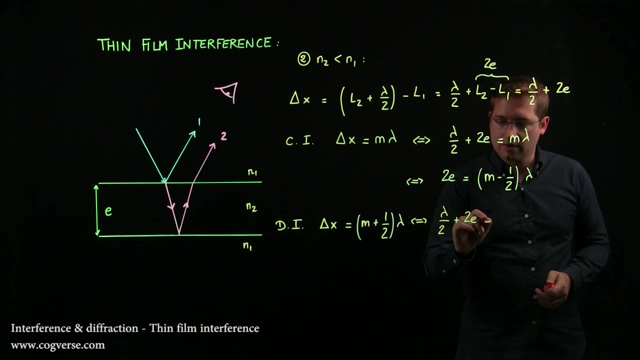 It is exactly the same thing. I just distributed the 2 of lambda over 2, basically- And this is the same as lambda over 2 plus 2e equals m plus 2e. So this gives me 1 half of lambda. 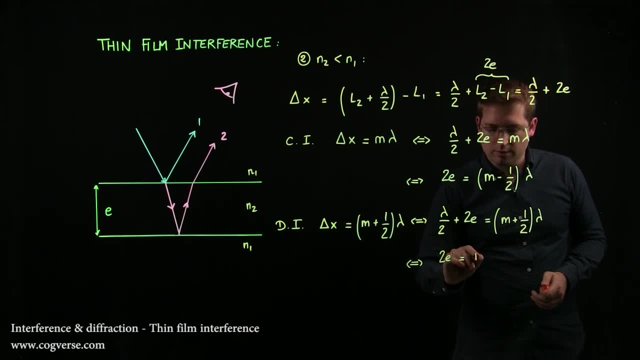 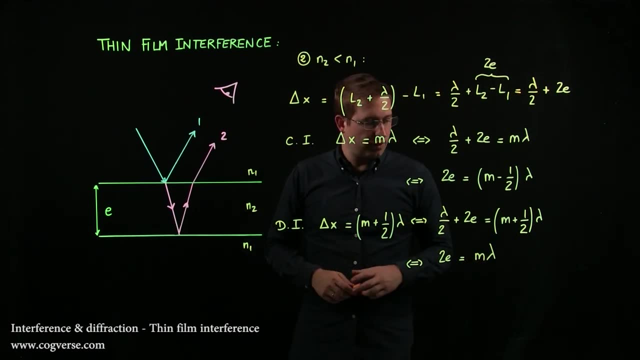 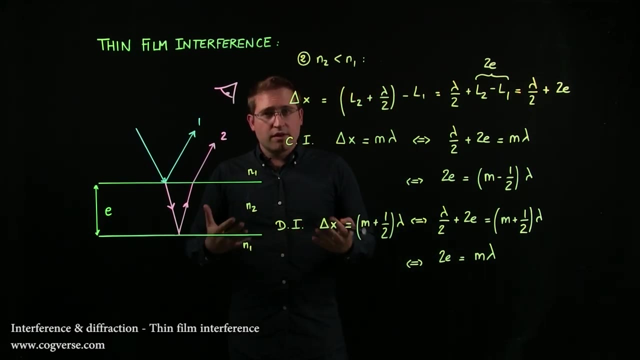 which is the same as 2e, is equal to m lambda And that gives you destructive interference. Any wavelength that satisfies this gives you destructive interference. So this is thin film interference. You need to understand how we set up delta x and accounted for the different phase shifts. 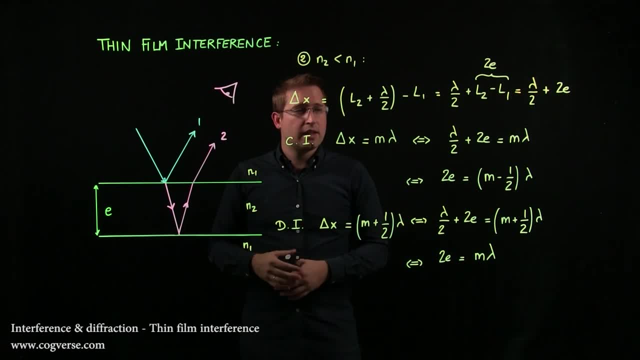 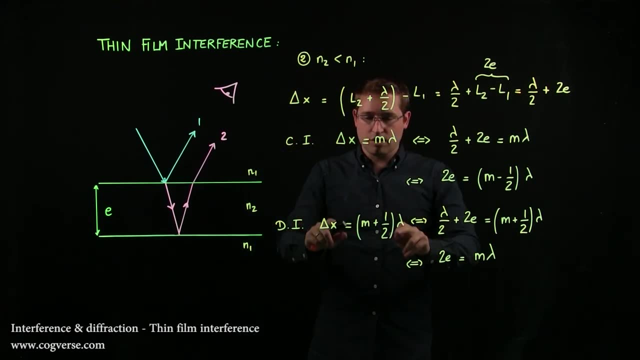 You need to know when there are phase shifts and when there are not, And you need to remember that the conditions for constructive interference and destructive interference are given here, And whether your end result looks like it's destructive interference although you want it constructive.